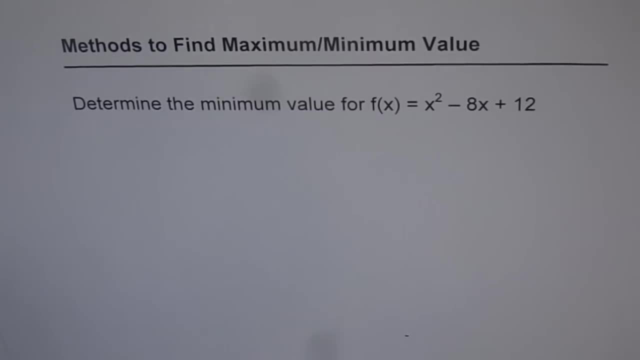 Methods to find maximum or minimum value. Determine the minimum value of the function x squared minus 8x plus 12.. Now in this video, I will explain you how to use different methods to find extreme value of a parabola, So a parabola represented by a quadratic equation. 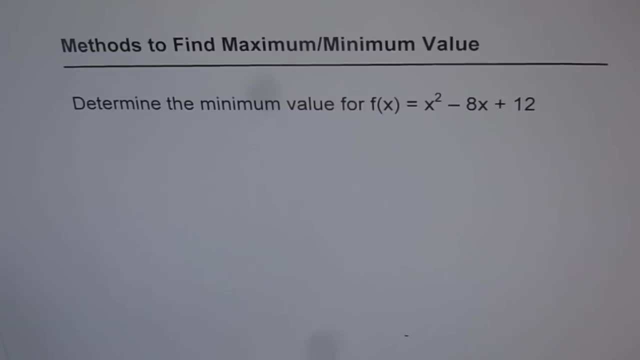 will always have a turning point and at that turning point it will be either a maximum or absolute minimum value. If the parabola opens up, then it has a minimum value, and if it opens downwards, then it has a maximum value. Now, when a given equation is like x squared, 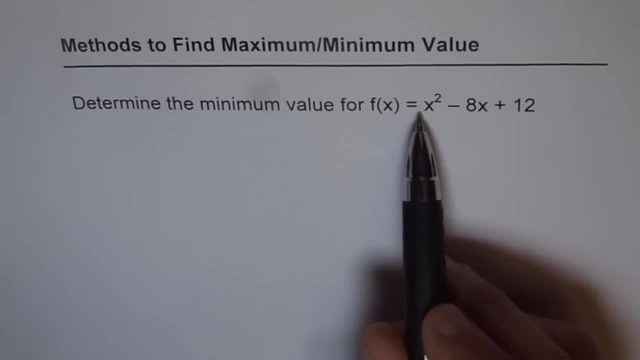 minus 8x plus 12, the coefficient of x is positive. Since it is positive, it opens up and it will have a minimum value. So in this case, we will find minimum value using a couple of methods. One of them is the vertex form. To convert it into vertex form, what we 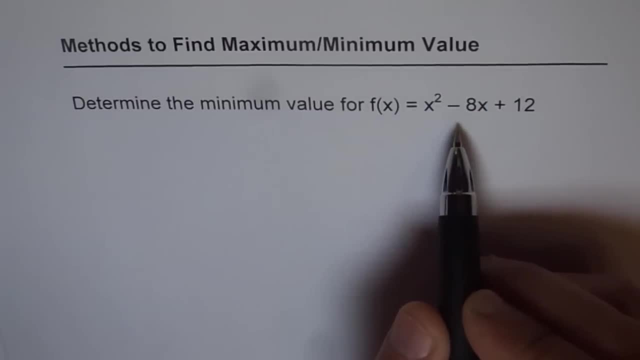 do is we kind of make it a perfect square. So let's go through the process. So the equation is x squared minus 8x plus 12.. We work with these two numbers. So I am putting a square bracket here to show that we are going to work with these two numbers and keep 12 on. 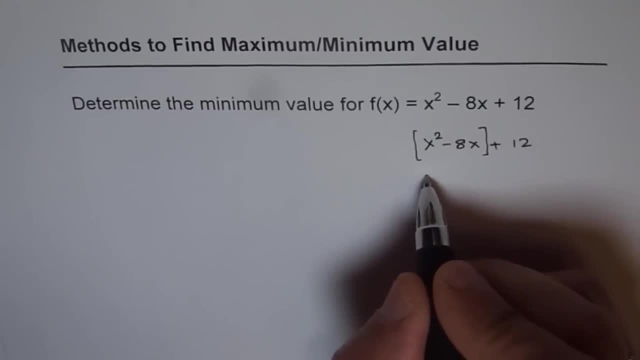 the side for the moment. Now the next step is that do half of this number 8.. So I am going to do half of this number 8, which is the coefficient of x. So half of 8 is 4.. Square it and subtract the same number minus 4 squared. So what we do here in the next step is we: 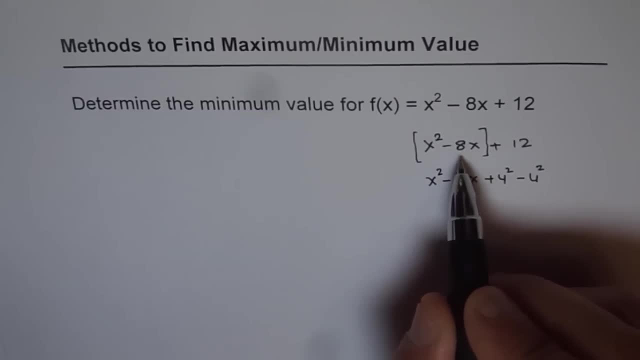 do half of the coefficient of x and square that number. Half of 8 is 4 and 4 squared is the number which we add and subtract. When you add and subtract the same number, you are not changing the equation, right. It remains the same. It is as if you are adding a zero. 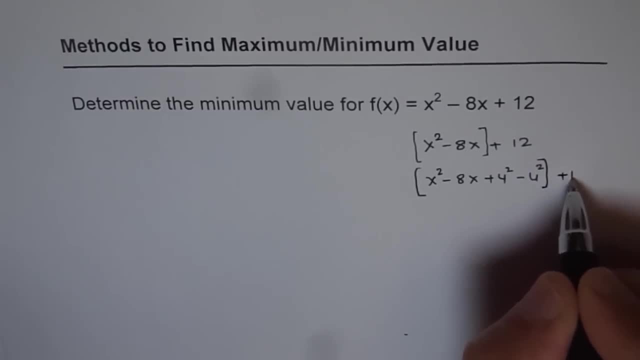 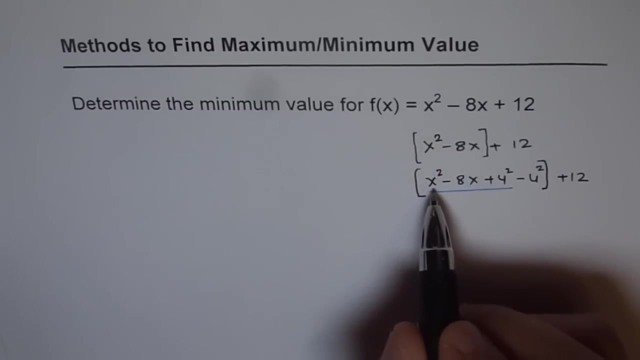 right, Let's put them in a square bracket and keep 12 on the side. Now you will see that the first three terms, that is, x squared minus 8x plus 4 squared, forms a perfect square. So this is a trinomial where the first term is x squared, the middle term is twice x and 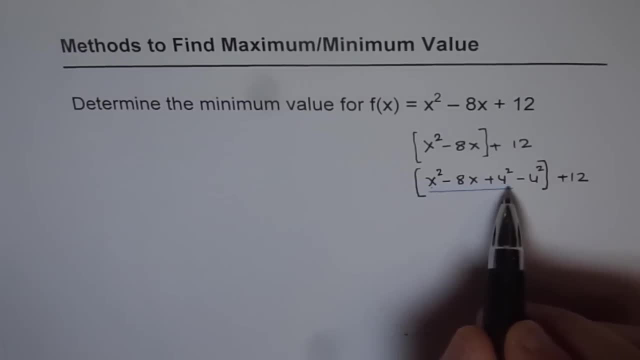 4, and the third term is 4 squared. So it forms a perfect square. So we can write this as x minus sign from here and 4 from the other side Square. So these three terms become x minus 4, whole square minus, we have 4 squared. Let me write this as 16. now 4 squared is. 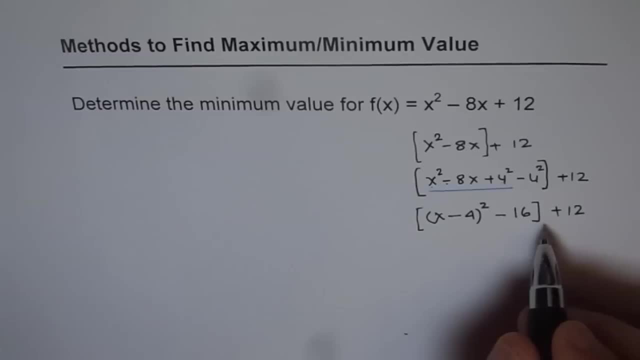 16 plus 12.. Now we can open the bracket and write down this equation in vertex form. It is x minus 4, whole square, and combine these two terms Minus 16 plus 12 gives us minus 4.. Now this equation is in the vertex form, and from here we know what the vertex is. 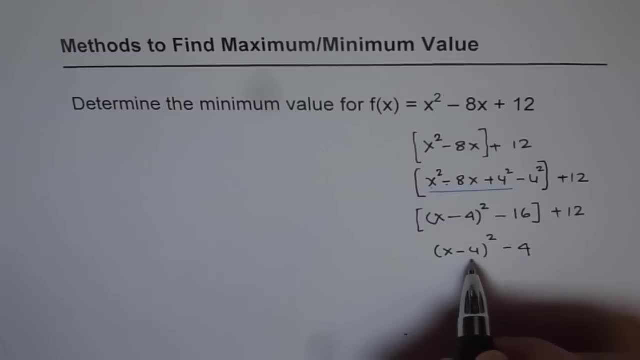 Vertex in this case is at 4 and the minimum value is minus 4.. So the vertex here is 4, with a minimum value of minus 4.. So the question here was: determine the minimum value of the function. So the minimum value of the function is minus 4, right, So what we did was we took. 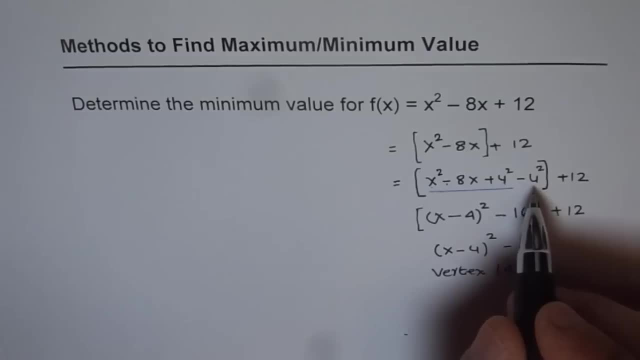 our function, added and subtracted square of half of b, the coefficient of x. Do you see that It helped to make a perfect square? and then we had the equation in the vertex form. This method is called completing the squares method. right, Let me write down the 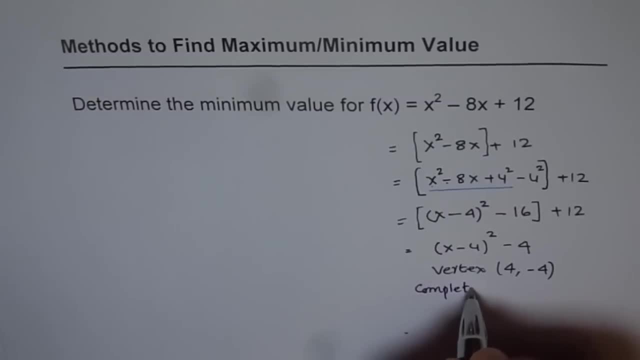 name: completing the squares: Complete squares. With this method we do get vertex and you can see the number of steps. This was simpler since the coefficient of x was 1.. If this would have been not 1 but some other number, in the first step we would have factored that out. So as a very simple example, I am. 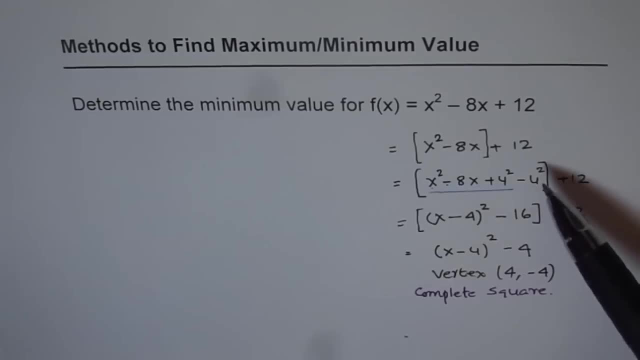 trying to demonstrate here different methods. We will look into more completing the squares details in coming videos. Well, let me answer this question first, and that is: minimum value is minus 4 right now. as you can see here, this is a parabola which will be opening upwards and the 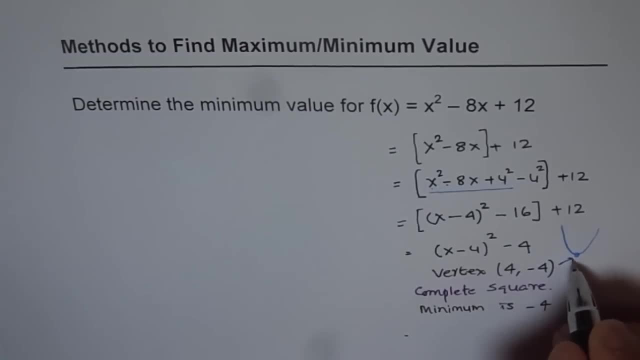 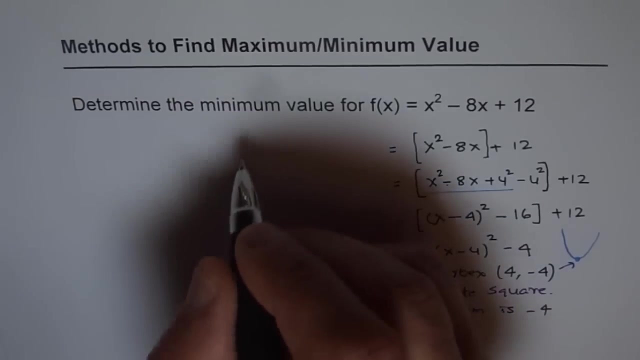 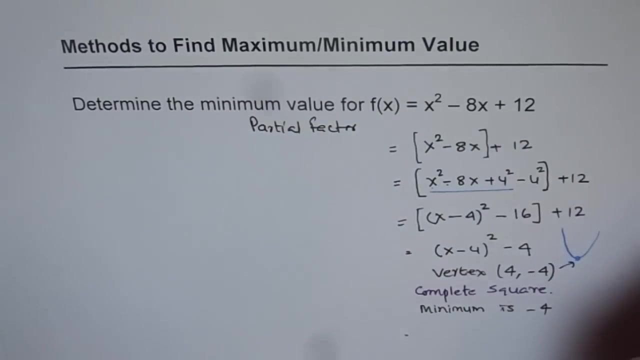 vertex will be as defined here. okay, since it opens upwards, we have a minimum value. now let's look into some other methods to find the minimum. and now i'll introduce you to a method which is called partial factoring. in partial factoring we do not factor the whole term, we just factor the first two terms. 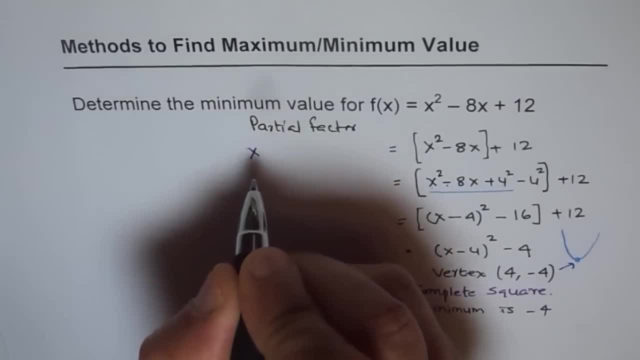 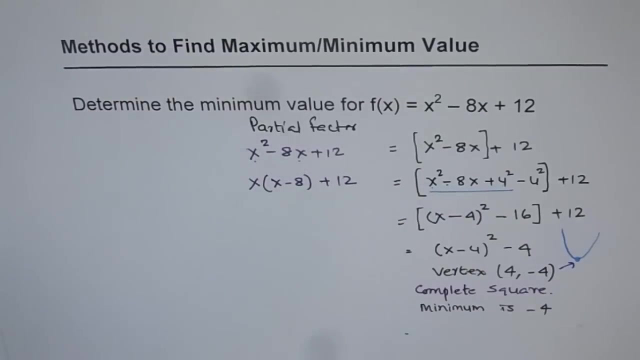 and let's see how it works. we are given trinomial fx equals to x square minus 8x plus 12. i can factor just these two and then write this as x and we are left with x minus 8 plus 12. right, as you can see here, it really means that at two points where x is 0 or x equals to 8, the 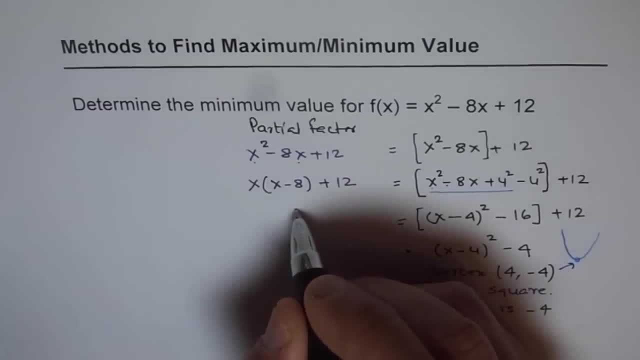 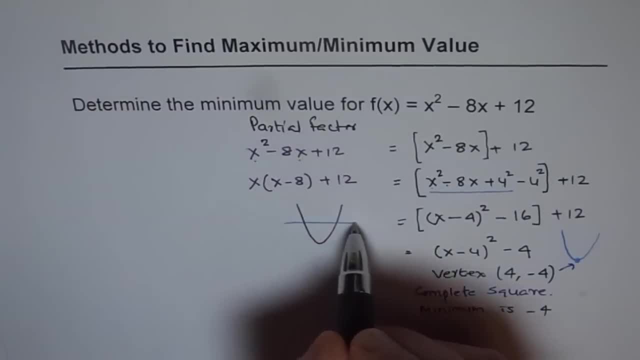 like this right. so you'll find if you draw a horizontal line right. so in this particular case, you will find that at x equals to 0 and at x equals to 8, the value of the function will be 12. do you understand this? horizontal line will give you the value of the function at x equals. 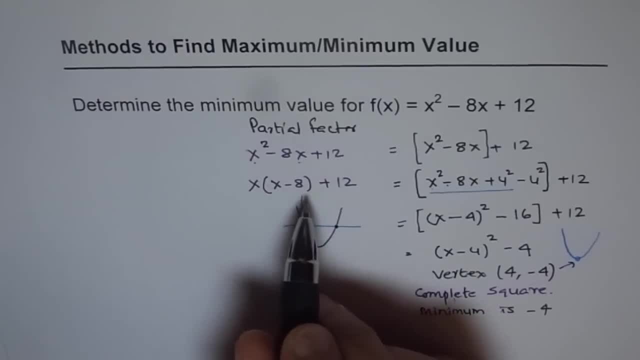 to 0 and at x equals to 8. now axis of symmetry will be right in between that line. do you understand axis of symmetry? every parabola will have an axis of symmetry and the meaning of axis of symmetry is that the points on the either side are symmetry. if you draw a horizontal line, that means: 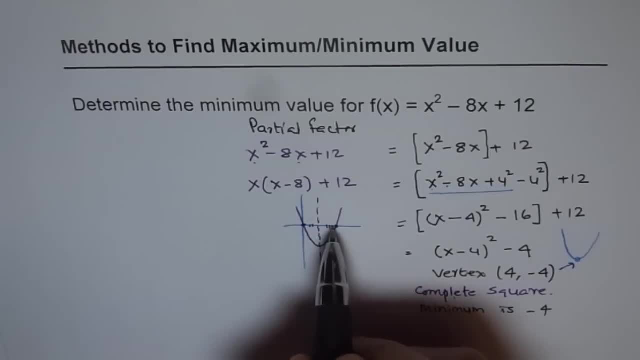 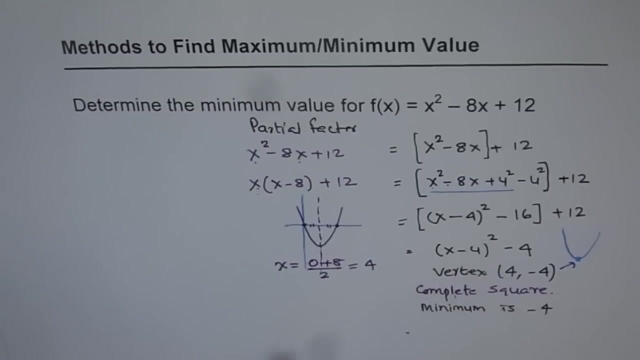 that that our vertex will lie in the center of these two points, right? So the center should be at a value which is midway between 0 and 8, correct? So if I find a point, x equals to 0 plus 8 divided by 2, which is 4 for us. 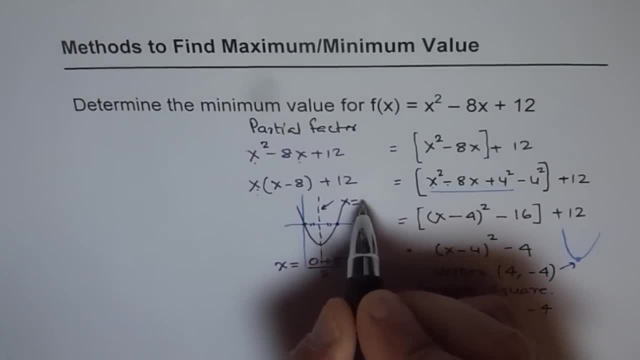 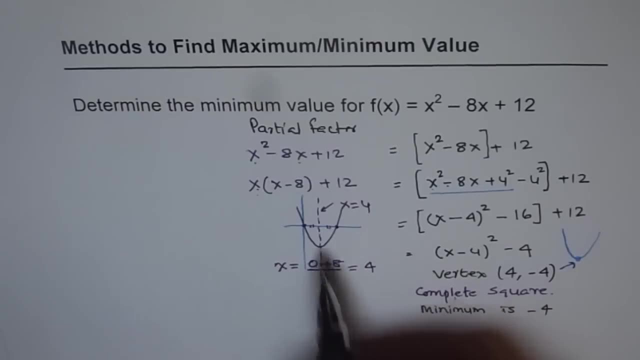 I know equation of x equals symmetry is x equals to 4.. And therefore I also know that at x equals to 4, we have a minimum in this case. Do you see? So we came to the same result: At x equals to 4, we have a minimum. 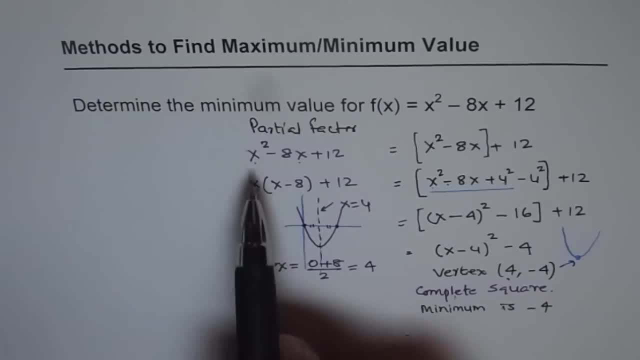 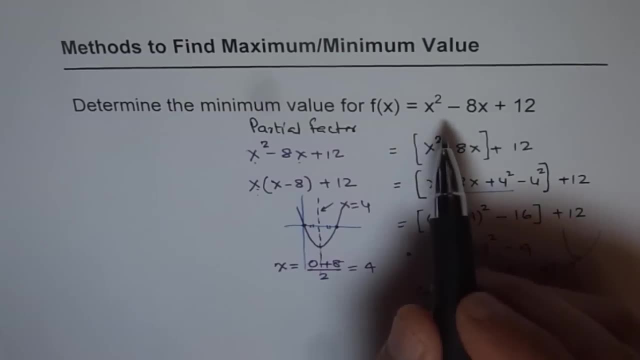 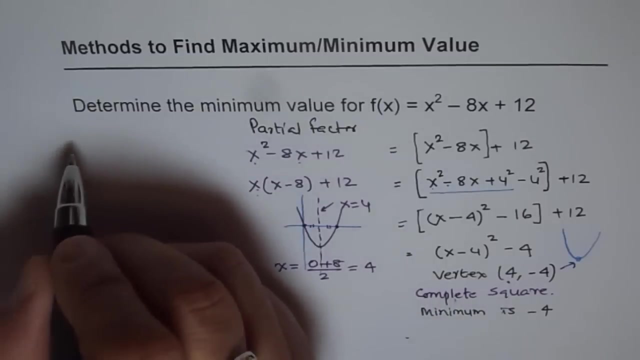 So we could have arrived at this value so fast using partial factoring. Now, one more method is that if you are given an equation in standard form, then you can use a formula. That is always. if I have a general equation, let us say ax squared plus bx plus c. 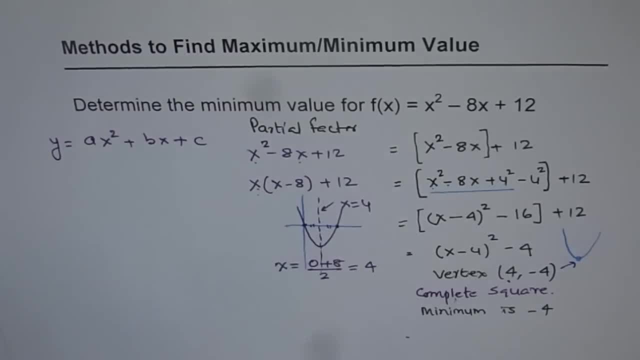 Let us say y equals to ax squared Plus bx plus c. This is quadratic function in standard form. Now here, what is the point at which you'll have maximum or minimum? The point will be at: x equals to minus b by 2a. 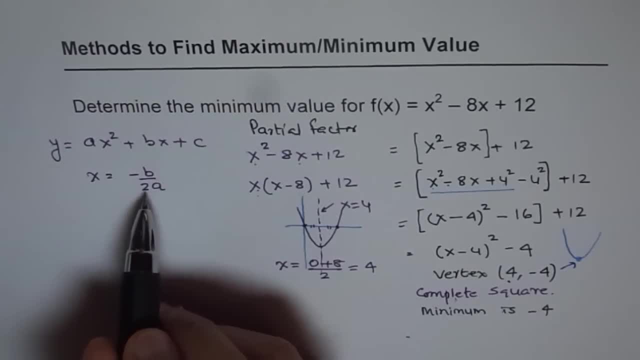 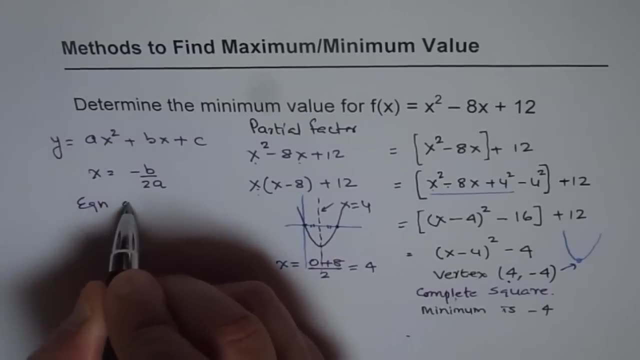 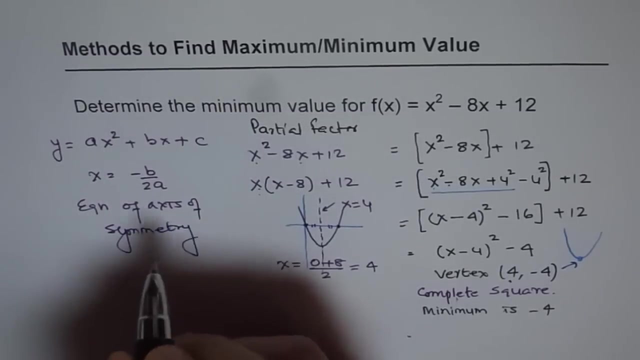 So at x equals to minus b by 2a, always we will have maximum or minimum. In fact, x equals to minus b by 2a is equation of axis of symmetry. Now, once you know the point, you can always plug in the value and find the answer. 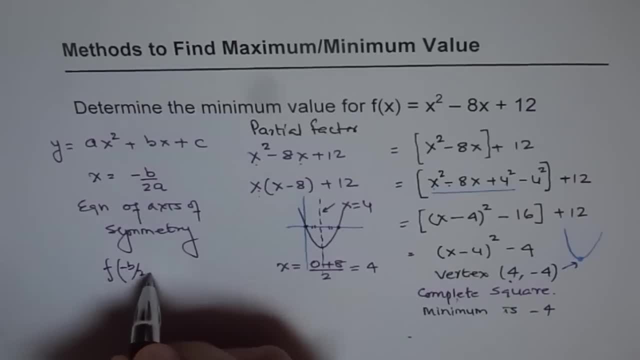 That means f of the value of function at minus b by 2a will be your maxima or minima, depending on a, whether it opens up or down, whether it is negative or positive. Do you understand? So that is how we can quickly find the point where maximum value or minimum value will lie. 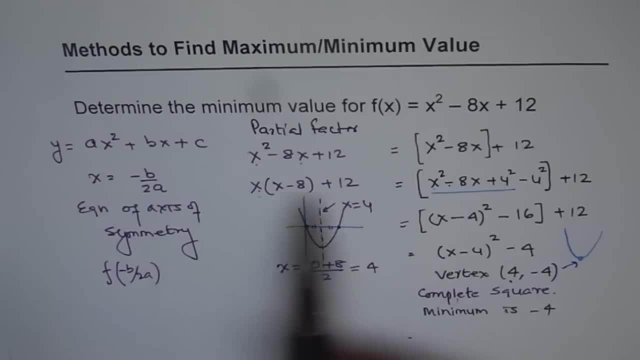 or axis of symmetry exists, Do you understand? So these are a couple of ways in which we can do, And, of course, you can always factor it correct. This one was easy factoring, So we could have factored this also. 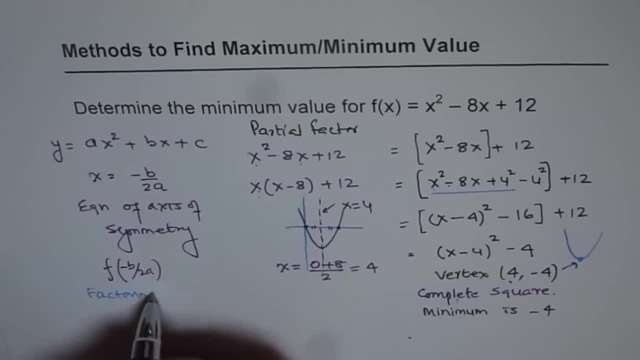 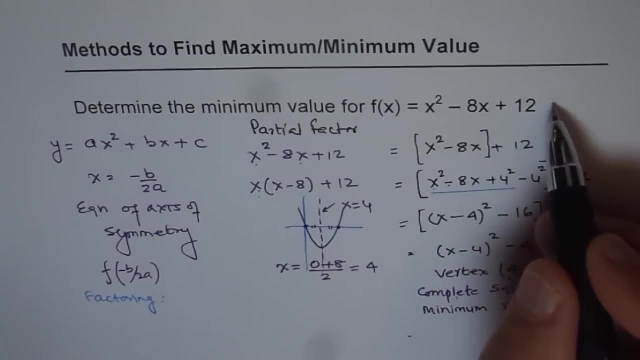 So the last is factoring, And I could have written this function in the factored form. We're looking for two numbers, whose product is 12, and whose sum is minus 8. So the numbers are 6 and 2,, right. 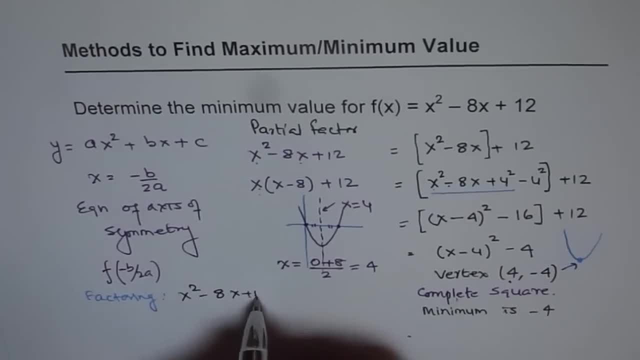 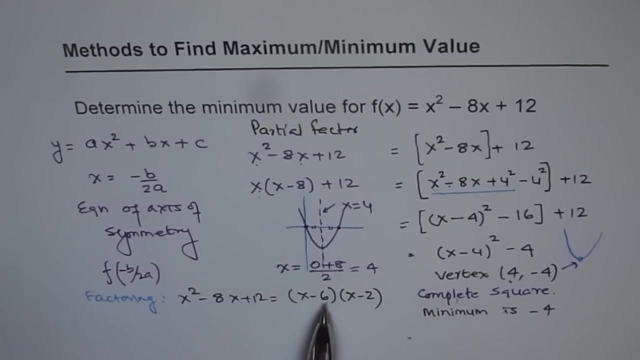 So I could have written: x squared minus 8x plus 12 equals to x. Now we need Minus, so both should be negative, right, And product is positive minus 6 times x minus 2.. So once you have your equation in factored form, then you know where the maxima or minima lies. 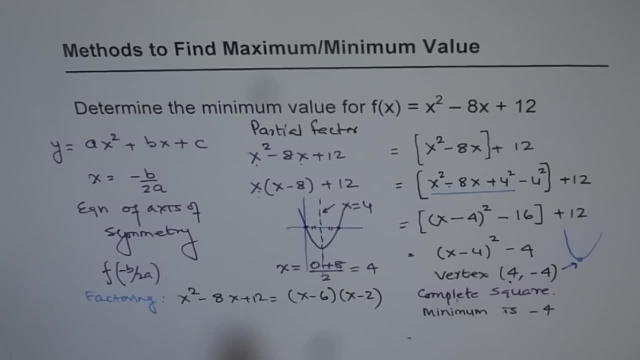 Well, this is positive. so we are looking for a minimum, and that should be in between the two factors, That is, 6 plus 2 divided by 2, which is 8 divided by 2, which is again 4..